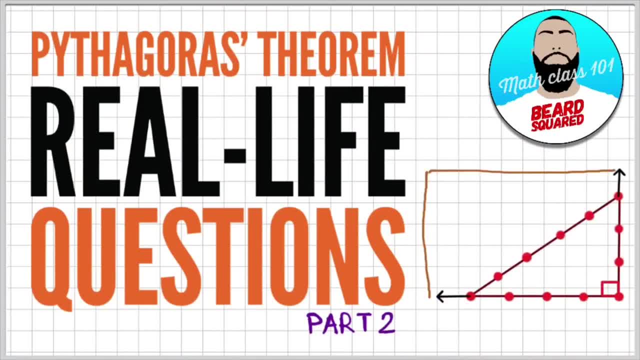 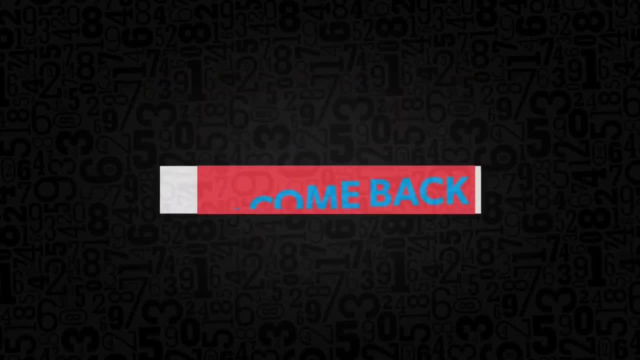 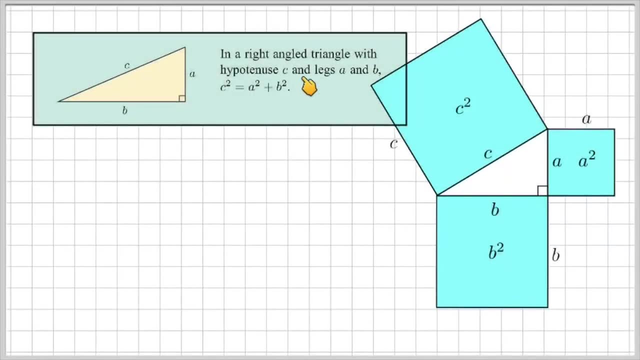 Hey, welcome back to Beard Squared. In this video we're going to be problem-solving real-life application questions using the Pythagorean theorem. Coming up In a right-angled triangle with hypotenuse C and legs A and B, we have the formula C squared is: 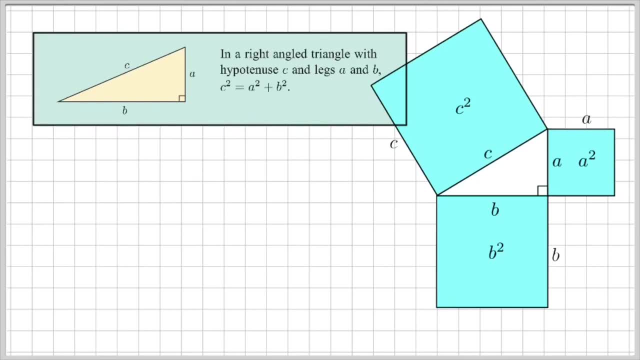 equal to A squared plus B squared. Now, if you have no idea what I'm talking about, I really do encourage you to go watch part one so you get a better understanding of Pythagorean theorem, and then we can move on to real-life application questions. So let's look at a problem We have. 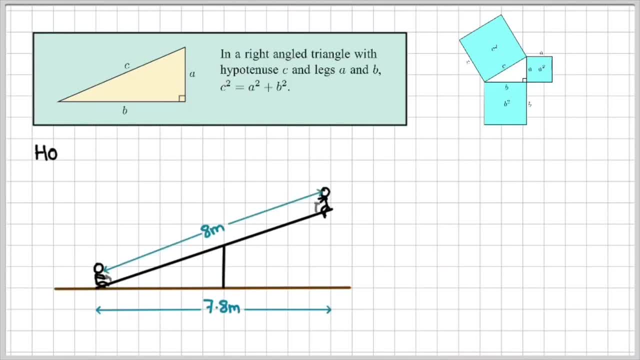 Jason and his sister in the park and they're playing on the seesaw, and what we want to find out is: how high does a child on the seesaw go? We know that we've got 7.8 meters across and that the seesaw is 8 meters long. What we need to find out is the height of the seesaw. 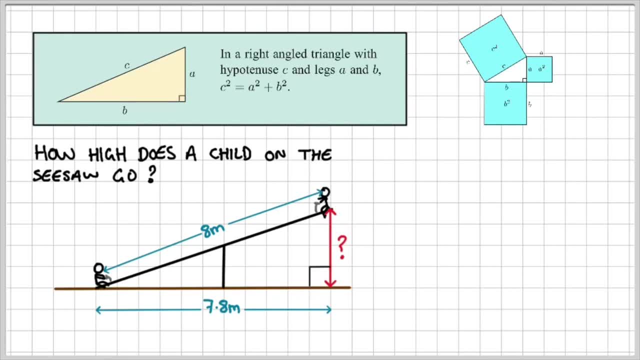 We can set this up because we know that we have a right-angled triangle. So we're going to use Pythagoras' theorem and if I label this, I know that opposite the right angle is my hypotenuse. So that's going to be my C and the other two sides are going to be A and B. Okay, it doesn't. 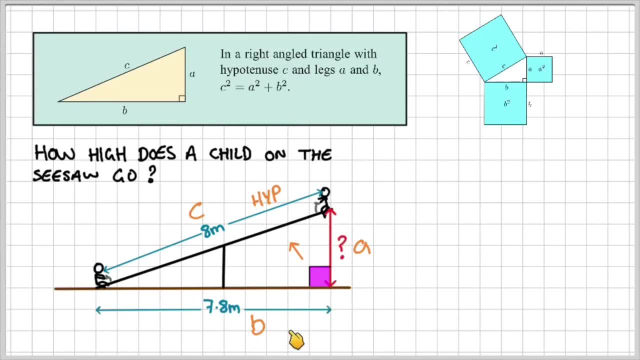 really matter which one's A, which one's B, but we can label them A and B. So now, if I set up the equation, I can say: A squared plus 7.8 squared is equal to 8 squared, and if I tidy that up, A squared plus 60.84 is equal to 64.. 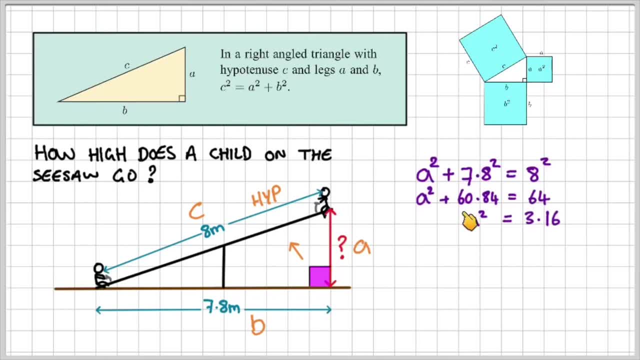 So if I rearrange that, 64 minus 60.84 would give us 3.16.. So therefore, A would equal to the square root of 3.16.. So remember we're only taking the positive square root of 3.16. 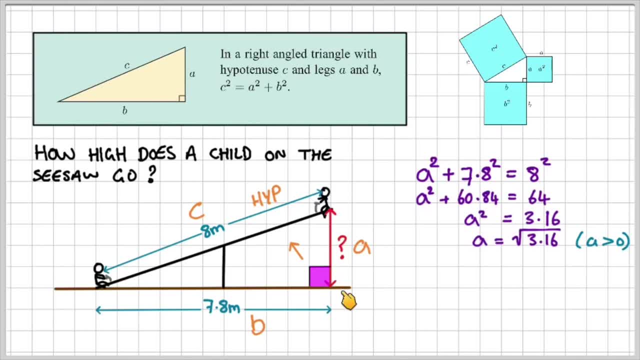 because A is going to be greater than 0. This is going to be a positive value. So if we find the square root of 3.16, we can therefore say: a child goes about 1.78 meters above the ground. 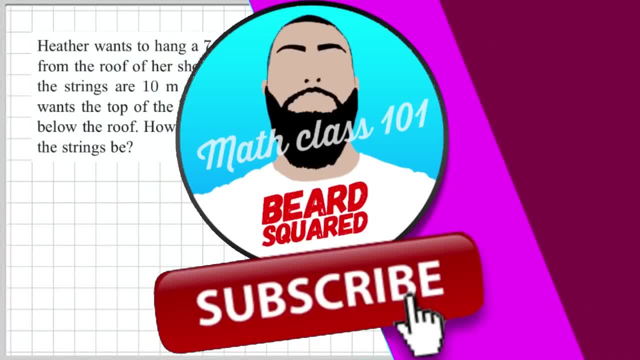 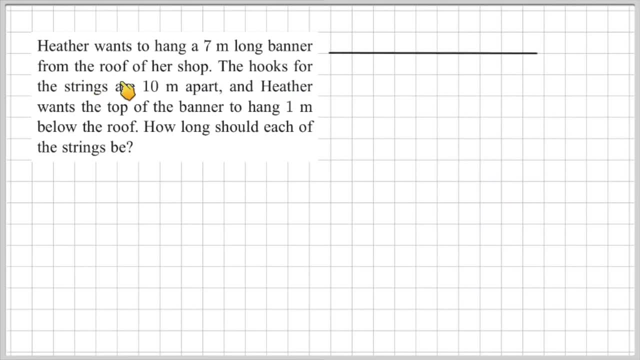 So now that you've warmed up and you've got a solid grip on Pythagoras' theorem, let's get our teeth stuck into it. So here's a problem. then It says: Heather wants to hang a 7 meter long banner from the roof of her shop. 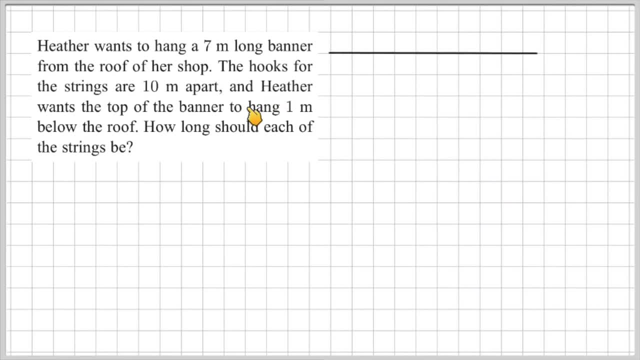 The hooks for the strings are 10 meters apart And Heather wants the top of the banner to hang 1 meter below the roof. The question is: how long should each of the strings be? So I've drawn a diagram of the banner, which is 7 meters long and the hooks are 10 meters apart. 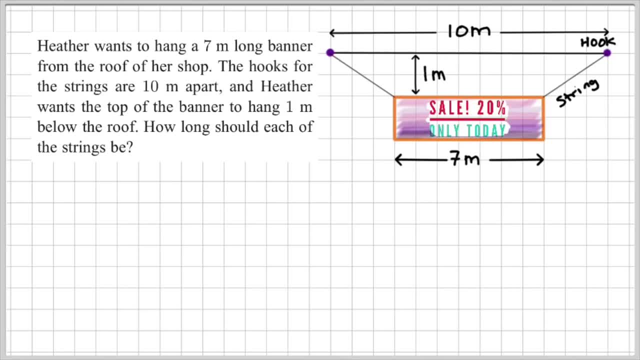 And Heather wants a sign to hang 1 meter from the roof. So what we know from the question is that the banner is 7 meters long. That means that this part here would also be 7 meters, which leaves a little gap here. 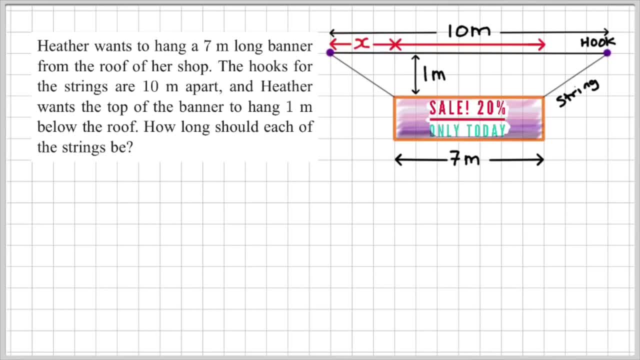 and here, And so I can label that as x and x. And if I set up an equation, I could say: 7 plus 2x is equal to 10.. So have a look here then: This is 7, this is my x, and there's my x. 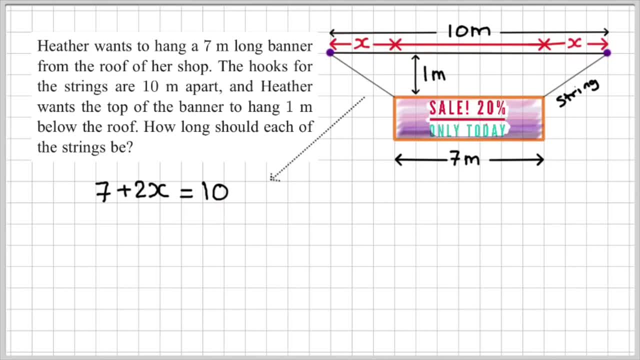 So 7 plus 2x is equal to 10.. Now I need to solve this equation to find out what x is, because if I find out what this x is, then I can set this up as a little right-angled triangle to find out what x is. 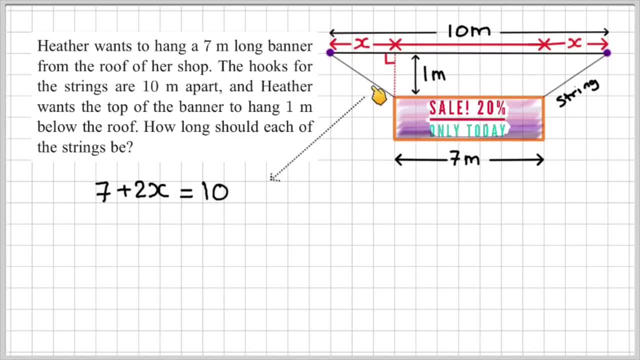 So let's find out what the hypotenuse is, and that would be the length of the string that we need. So let's solve this equation. So 10 minus a 7 would give us 3,, so 2x is equal to 3.. 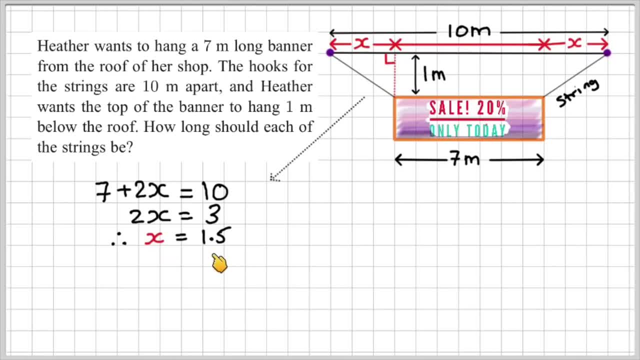 And then 3 divided by 2 would give us x equals to 1.5.. So now that I know what x is, I can set up my little right-angled triangle, which will give me x is 1.5, and the height, which is 1 meter. 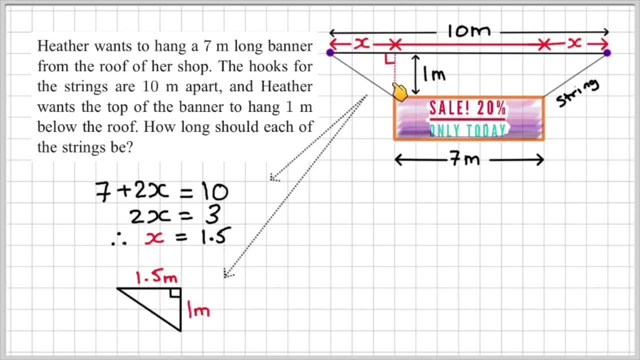 Now remember- I've just taken that information from here- This is my height of 1 meter and that's the x that I just worked out, which is 1.5.. Now remember, opposite my right angle is my hypotenuse, so that's going to be my c.